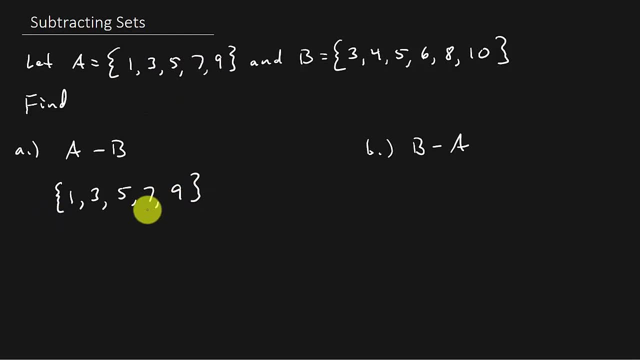 So there's set A. See that, Here's set A. So all I did, I just wrote it down again, All right, And then all you do is just go through set B, because we're taking out what's in B. 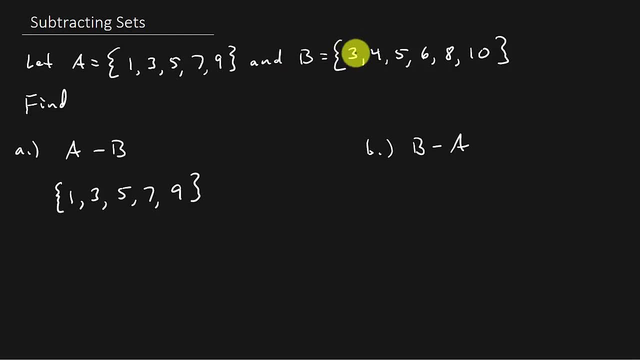 So do you see how? the element 3. Set B is in set B, so we have to take that one out And then we go to the next element, 4.. 4 is not in here, so we don't do anything. 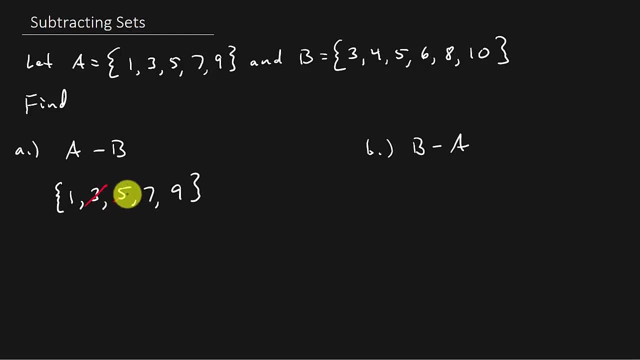 5.. Well, 5 is in here, so we have to take that one out. also, 6, it's not in here, 8's not in here, 10's not in here. So A minus B is equal to 1,, 7,, 9.. 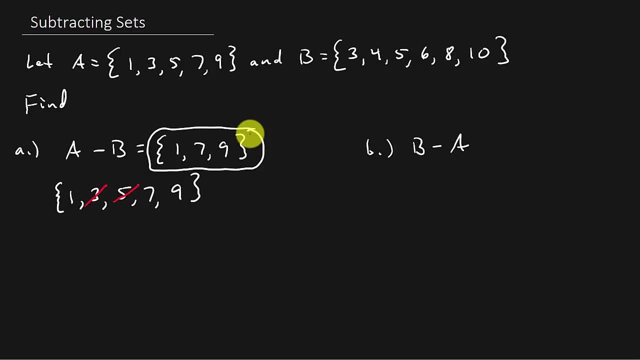 And that's your answer. So all you have to do is just write down this first set here and then take out the elements that are in this one. That's it. Let's do this: one B minus A. So just write down set B. 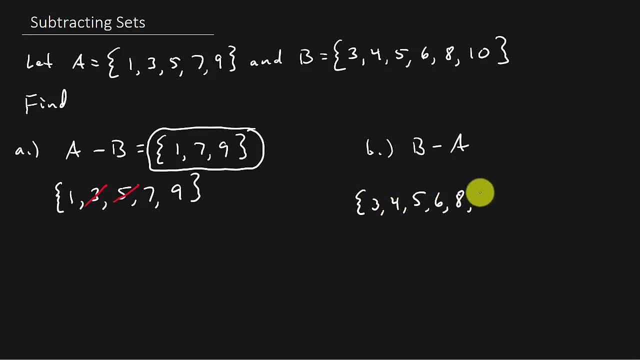 So that's 3,, 4,, 5,, 6,, 8, and 10.. All right, So here's set B. Now let's take out the elements that are in A. So let's see 1, not in here. 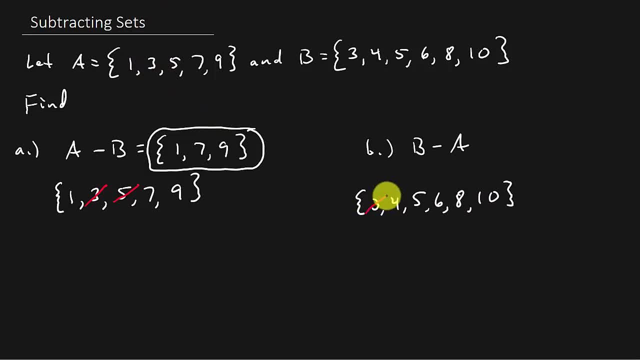 3, well, 3's in here, so let's take that one out. 5, well, 5's in here, so we take that one out. 7, 7's not in there. 9, 9's not in there. 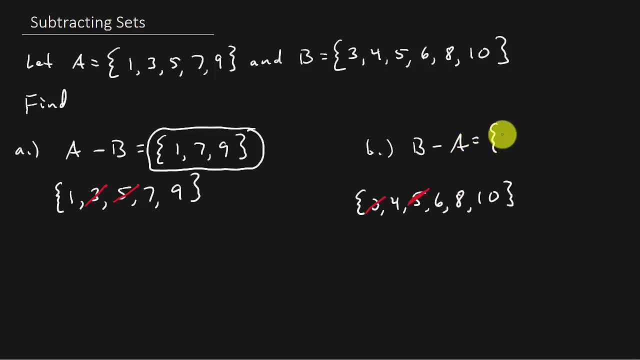 So our answer is 4,, 6,, 8,, 10.. And there's your answer, All right. So I hope that helped. Check out my other videos And the video for the sets on union intersection and complement. 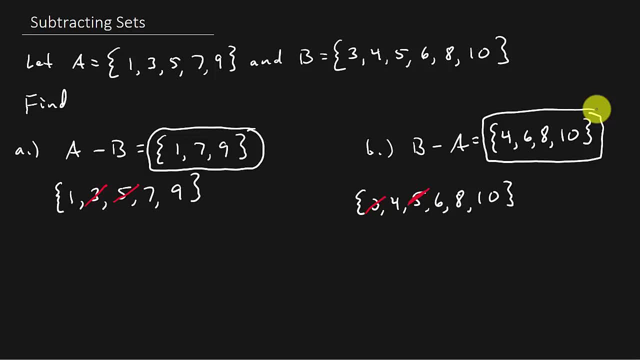 I'll leave a link to that one below. Thanks for watching. Give me a like, share and subscribe And I'll see you later.